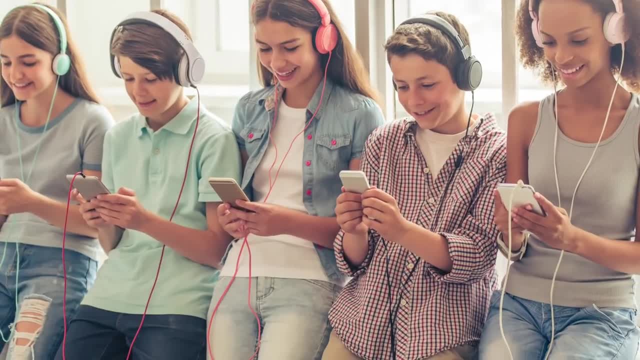 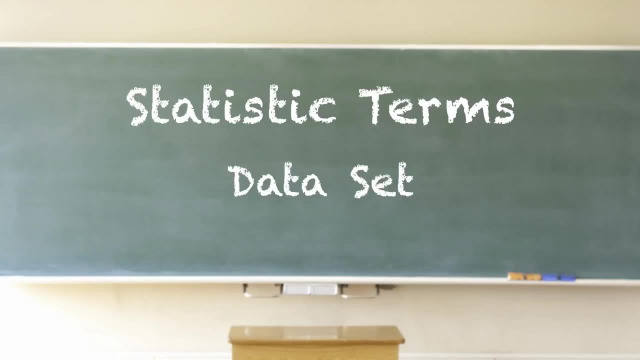 as well by saying. a lot of other people like this, so I will probably like it too. There are several important numbers used in basic statistics. The data set, the mean, the median, the mode and the range. Regardless of the data collected, every set of statistics usually has a. 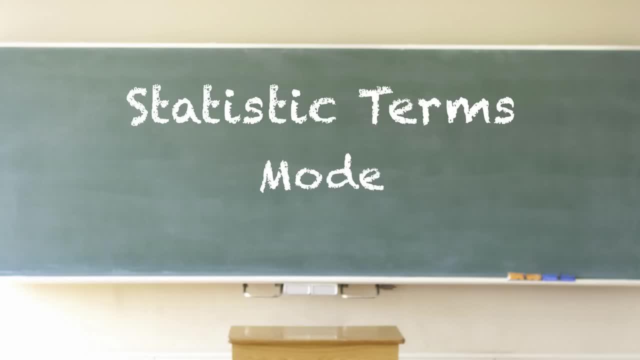 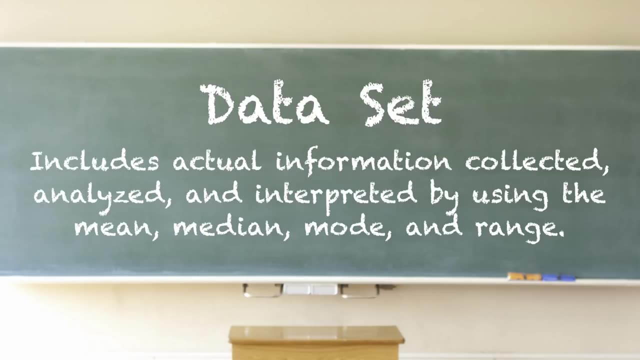 median and a range, and some sets will also include a mode. What are they? The term data set includes the actual information collected, analyzed and interpreted by using the mean, mean, median, mode and range. All statistics begin with a set of data, usually numbers. 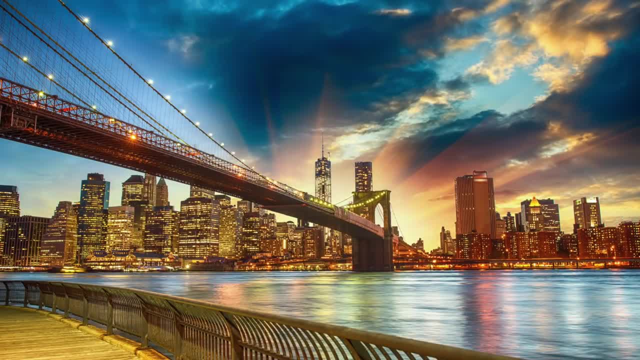 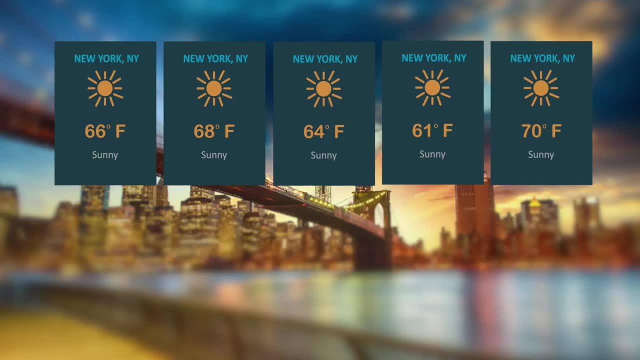 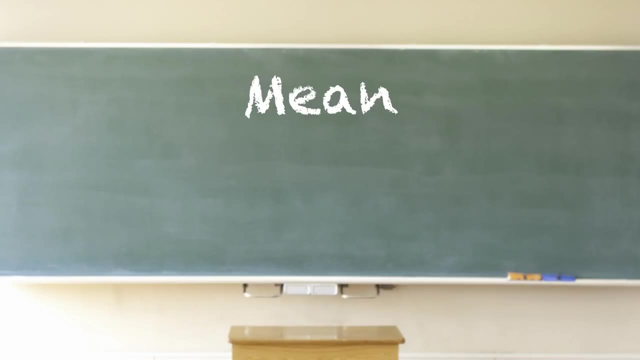 Here's an example. Ten straight days of temperatures in New York City during October were 66,, 68,, 64,, 61,, 70,, 72,, 72,, 68,, 64, and 64. Mean Most likely. you have heard the word average. 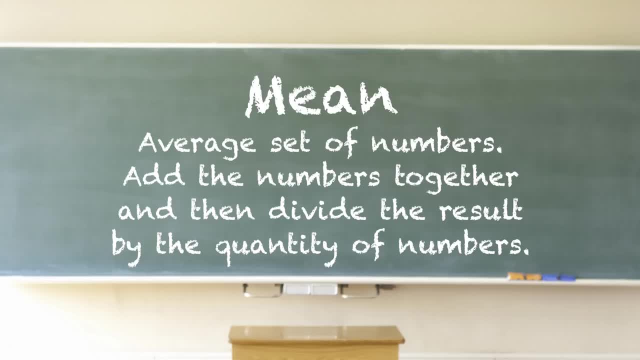 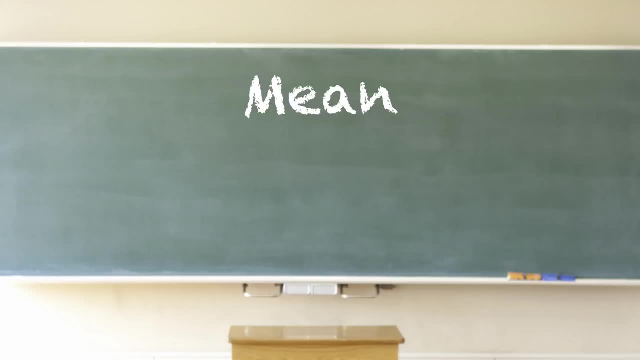 The mean is simply the average set of numbers. You add the numbers together and then divide the result by the quantity of numbers. For example, add the temperatures together and then divide by 10.. 669 divided by 10 equals 66.9.. 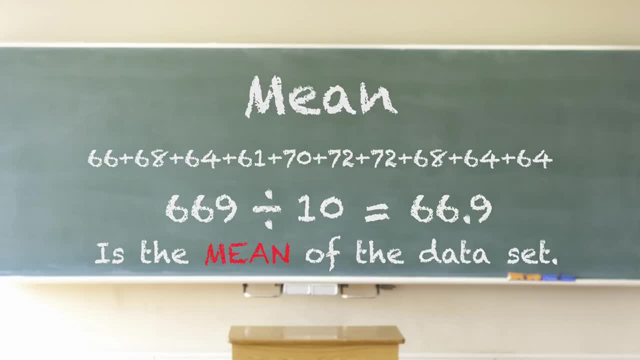 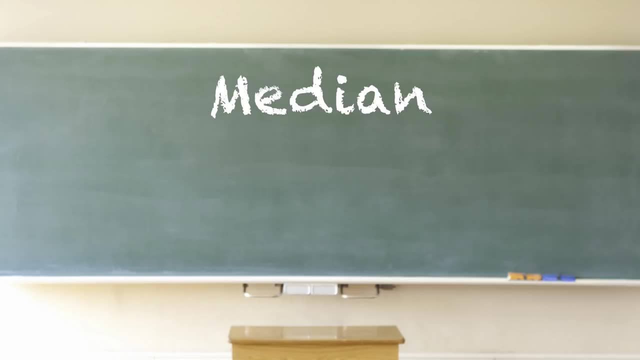 66.9 is the mean of the data set Median. The median of a set of data is the middle number of a set of data. To find the median, align the data from the smallest to the largest. If the quantity of numbers is even, add the two middle numbers together and then divide by 2.. 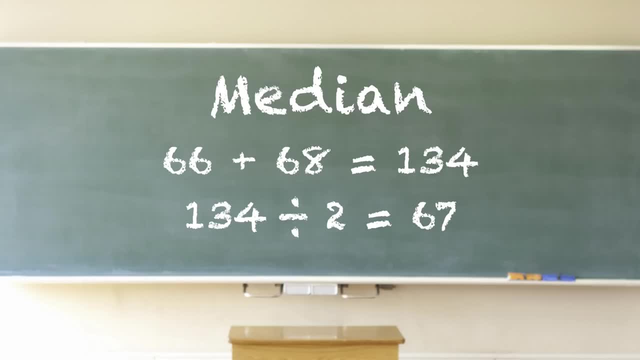 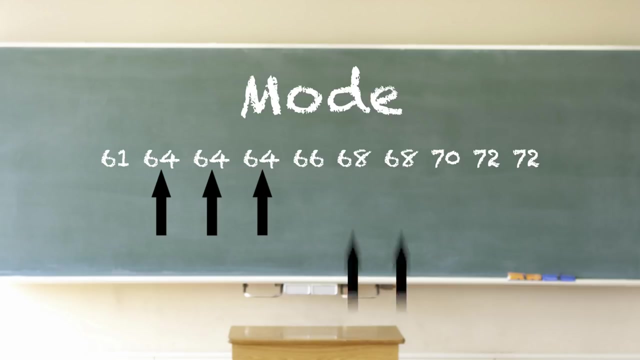 134 divided by 2 equals 67. So 67 is the median Mode. The mode for a set of data is the number appearing the most. If numbers appear an equal number of times, there could be more than one modes. 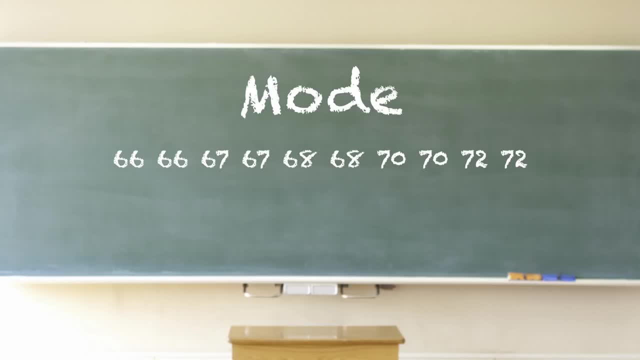 If every number appears an equal number of times, then there is no mode. The mode for a set of data is the number appearing the most. For example, use the aligned numbers. Which number appears the most? If you said 64,, you're right.